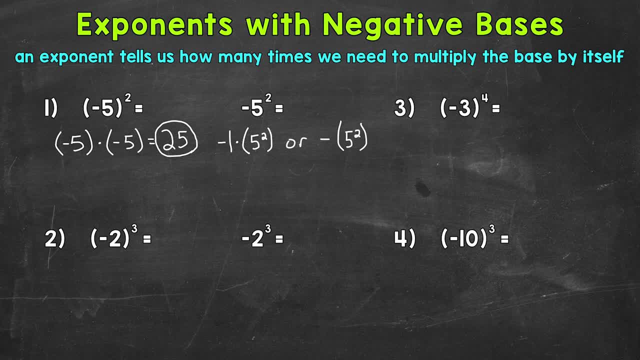 well, positive 5 times 5. 5 squared, that gives us 25.. we have to do that 5 squared first due to the order of operations that comes before multiplication. so 5 squared 5 times 5 equals a positive 25.. then we bring down our negative 1, so we have negative 1 times 25. well, a negative times. 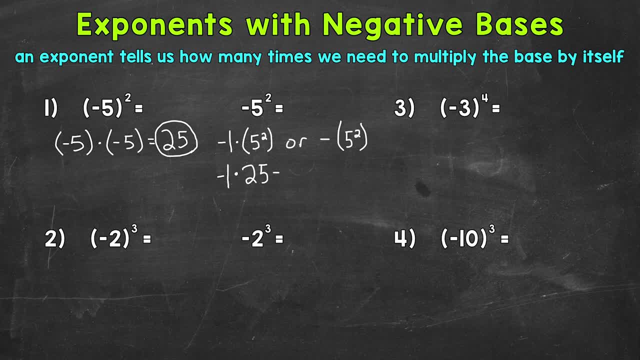 a positive equals a negative. so this is going to give us negative 25. that negative stays in front, or we can think of it as the negative staying in front here and we have 5 squared. we do that first and that negative again just stays in front. so 5 squared is 25 and then the negative. 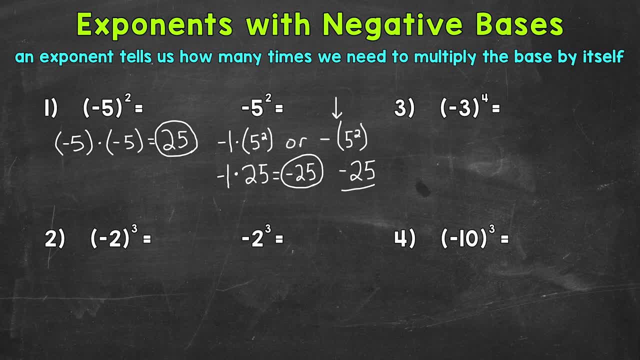 is not attached. it stays in front. so we get negative 25.. a couple different ways of thinking about it there, but the main point being the negative is not attached to that 5. it just stays in front. so our solution or answer here is going to be negative, no matter what. now, as 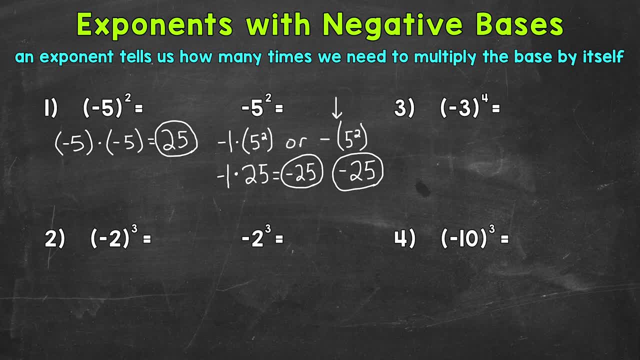 far as with the parentheses, if we have a negative times a negative, we end up with a positive. now, there are some cases where we will end up with a negative, no matter what, whether we have parentheses or no parentheses, and we are going to take a look at number two to see what that looks like. so let's. 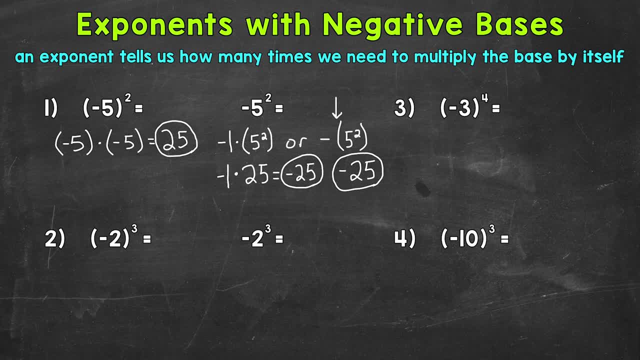 look at number two. let's take a look at where we have negative 2 cubed. so let's start with the one with parentheses. so the negative is attached to the two. so this means negative 2 times negative, 2 times negative 2.. let's write that out: so: negative 2 times negative, 2 times negative 2. 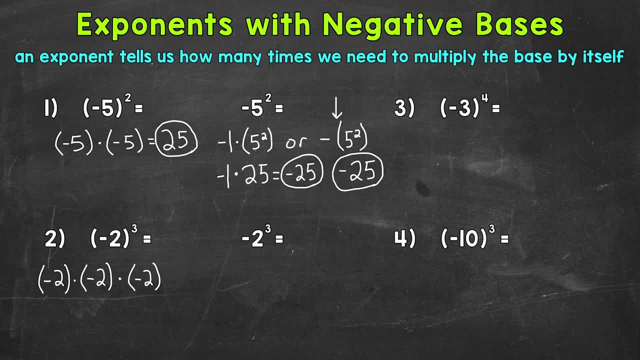 Negative 2 times negative: 2, well, a negative times a negative equals a positive. so we get a positive 4 here, And then we have one more negative 2, so a positive 4 times a negative- 2, well, a positive times a negative equals a negative. 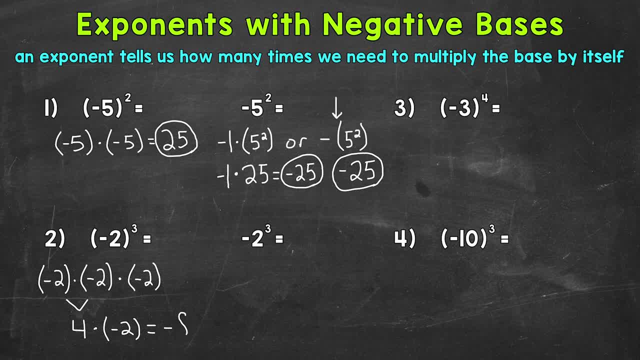 So this is going to give us negative 8.. Now for this one. we're going to get the same exact answer, without parentheses, because remember that negative is going to stay in front, so our solution or answer is going to automatically be negative. 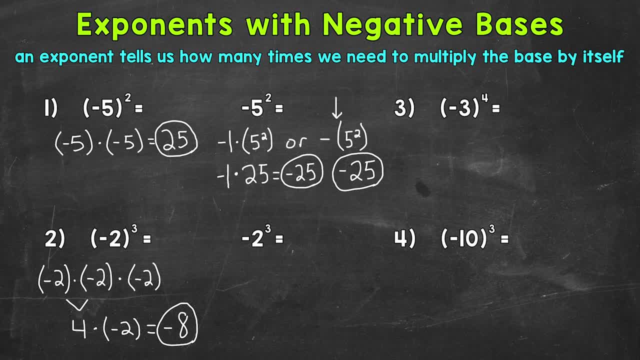 Let's see what that looks like. Essentially, what we have here is negative 1 times 2 cubed, a positive 2 cubed. The negative is not attached to the 2.. Well, a positive 2 cubed is 2 times 2 times 2.. 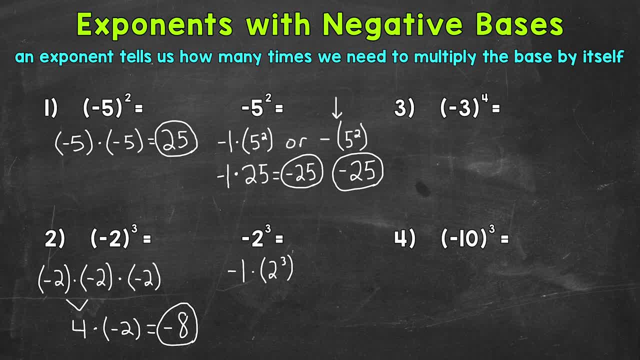 2 times 2 is 4, times 2 is a positive 8.. So a positive 8, and then we still have our negative 1 times that positive 8.. Well, a negative times a positive equals a negative, so we end up with negative 8.. 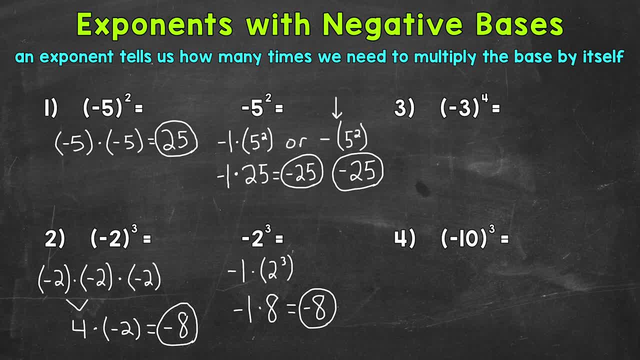 There as well. So in that case the parentheses do not impact our solution or answer, because it's going to be negative either way. Another way to think of that real quick would be leaving the negative in front. and then we have 2 cubed. 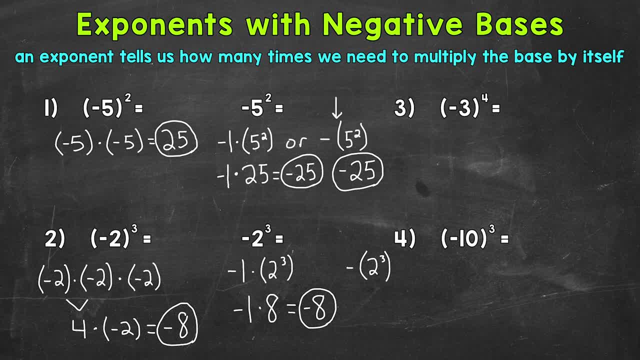 Remember the negative is not attached to that 2, so we have 2 cubed, which is 8.. And then that's. That negative is in front, so we end up with negative 8.. So a couple of different ways to think through that as far as leaving that negative sign in front. 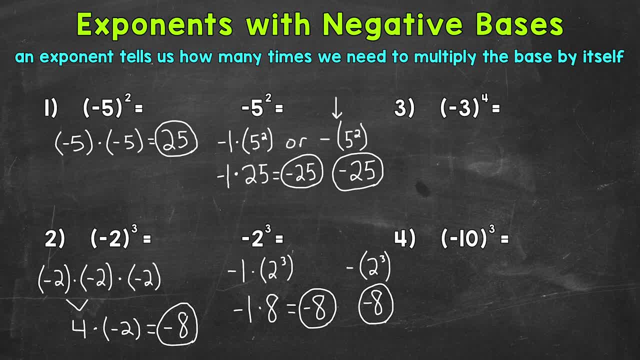 and we automatically get that negative solution or answer there. Let's move on to number 3, where we have negative 3 to the power of 4.. And the negative 3 is within parentheses, so the negative is attached to that 3.. 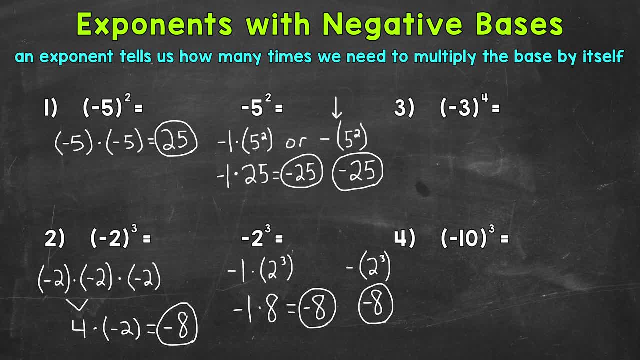 It's included with the 3.. So we have negative 3 times negative, 3 times negative, 3 times negative, 3.. So let's see what this equals. Well, negative, 3 times negative, 3.. A negative times a negative gives us a positive 9..